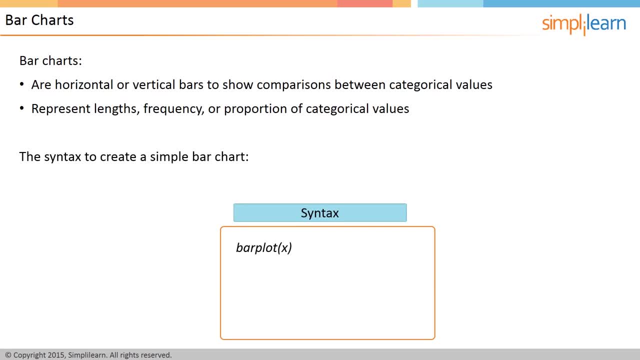 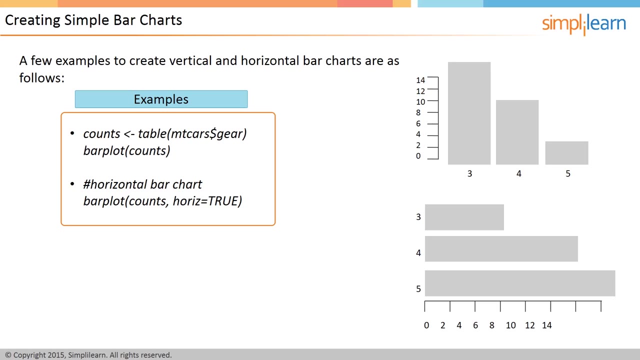 In the function matrix stands for height, which is a matrix or vector. If the height parameter is a vector, the values of the vector give the heights of the sequence of rectangular bars that make up the plot. Let us look at a few examples of how to create vertical and horizontal bar charts Here. 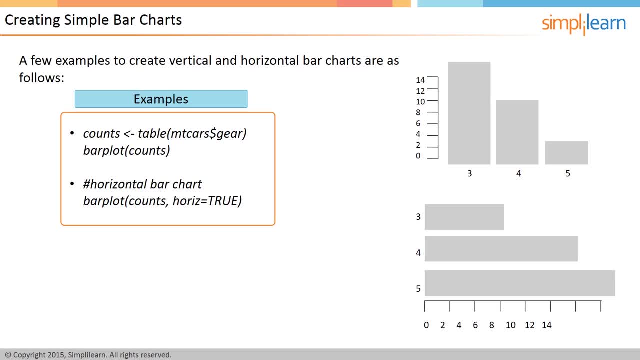 by using an embedded dataset of empty cars, you can plot bar graphs. To create the first bar graph, you pass gear data to the barplot function. The default setting for bar orientation is vertical. To plot a horizontal graph, you can pass horizontal equals true as the second parameter. 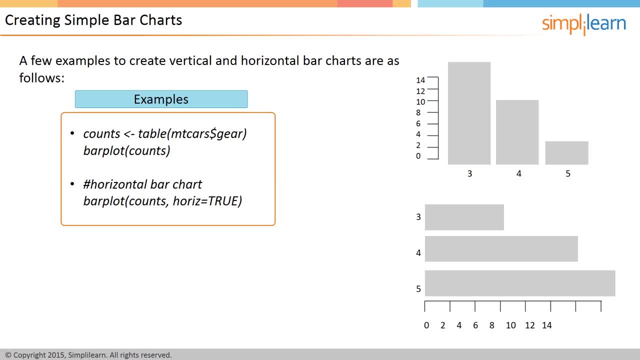 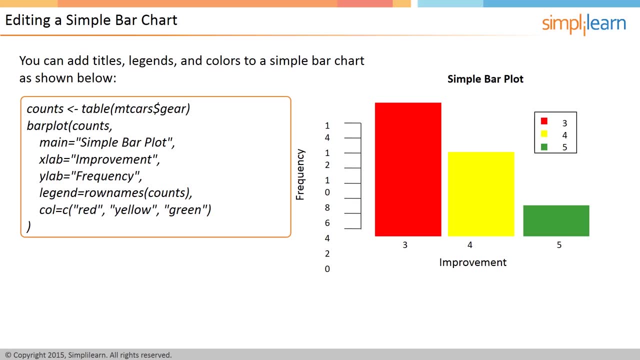 to the barplot function. In the next screen we will take a quick look at a few arguments to edit simple barplots. Here you can add labels, colors and titles to the barplot by using specific arguments. For example, legend is useful when the height is a matrix. The arguments x-lab and y-lab. provide the labels for the x-axis and y-axis respectively. You can also add a barplot to your script. Here you can add a set of arguments and you can add your own tests. And here is a simple approach to adding labels to the barplot. 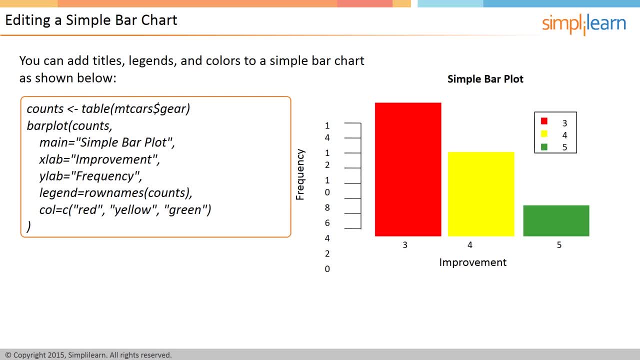 At least the somewhat straightforward approach is applied. Next screen is where you can add labels to. the Call will define the color of each bar By default. if height is a vector, then gray is used, whereas if height is a matrix, a gamma-corrected gray palette is used. 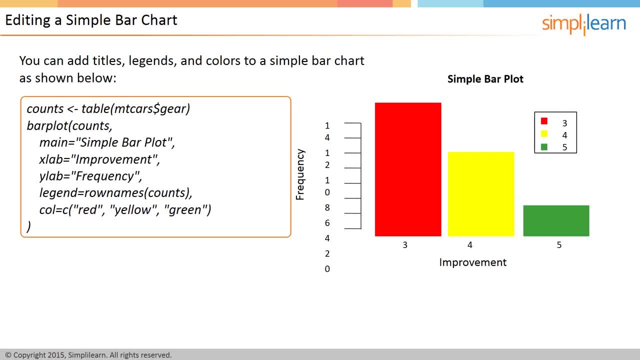 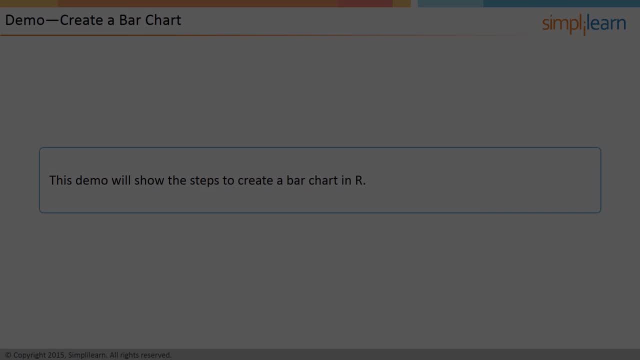 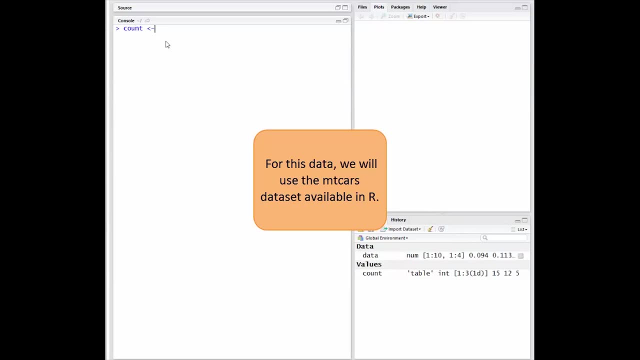 Main sub gives the overall and subtitles for the bar plot. This demo will show the steps to create a bar chart in R. In this demo, you'll learn how to create bar charts For this data. we will use the mtcars dataset available in R. 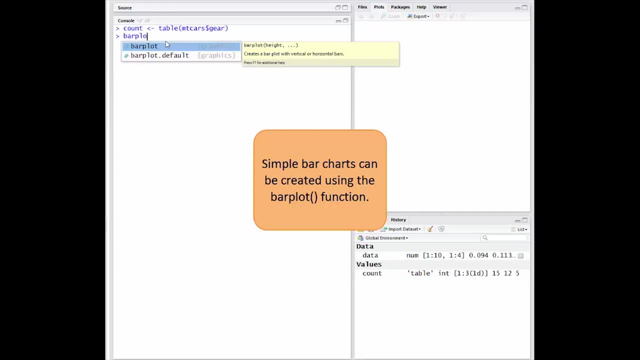 Simple bar charts can be created using the bar plot function. You can create horizontal bars by specifying horizontal equals true as an argument to the bar plot function. You can also add title colors and legends to bar plot by specifying details in an argument. 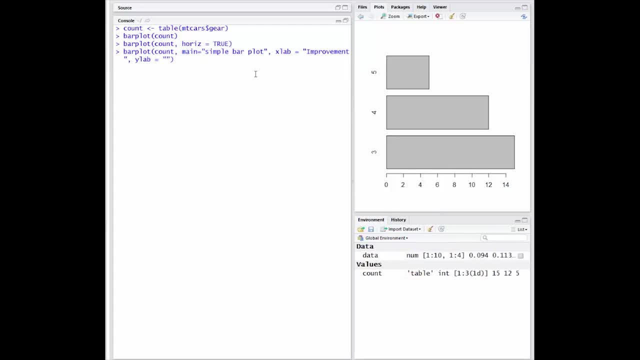 Here you'll see the bar chart bar chart. It's menu with the bar chart we'll be adding this time It'll also be if you want to add an object In the default bar chart, the bar chart bar. As you can see, the bar chart bar chart is completely automatic. 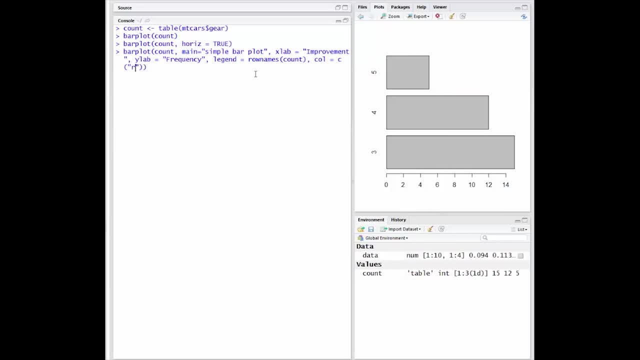 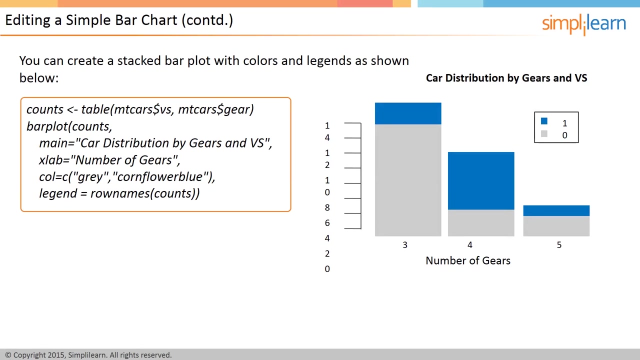 All you have to do is hit enter and select the bar chart. You'll see the bar chart. bar chart will pop up in the bar plot. For more options or help document, type the given command in the console. You can create a stacked bar plot if the input is a matrix. 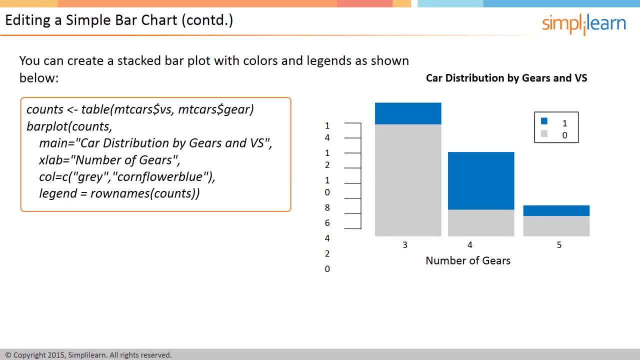 The stacked bar will indicate each column on the matrix. The argument Beside specifies if you want the bars to be stacked or adjacent to each other. By default, Beside is set to False and if Height is a matrix, a stacked bar graph results. 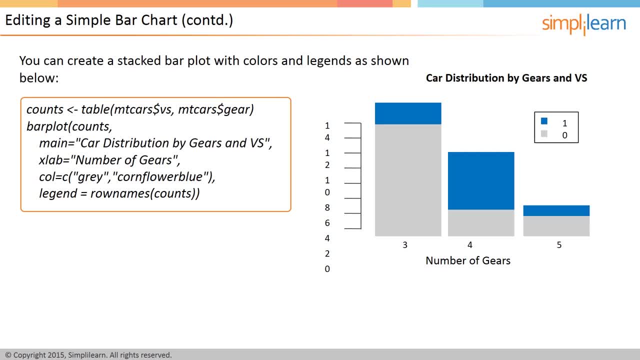 If you set Beside to True, then you get the columns of Height as adjacent bars. You can create a stacked bar plot with colors and legends, as shown in the screen. Here in this example on the screen it's a matrix of VS and Gear data from mtcars datasets. 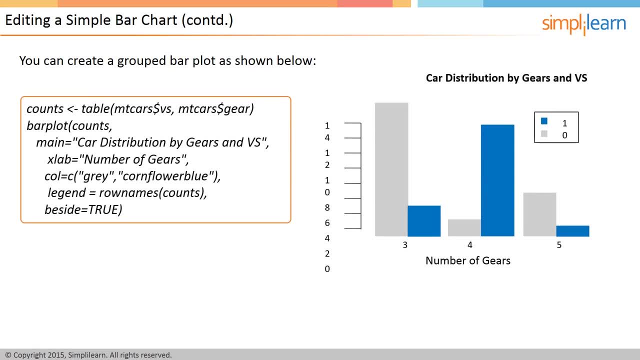 Using the same example as in the previous screen, you can create a grouped bar plot Reiterating. if the height parameter of bar plot function is a matrix and Beside is set to True, then the values in each column are juxtaposed rather than stacked. 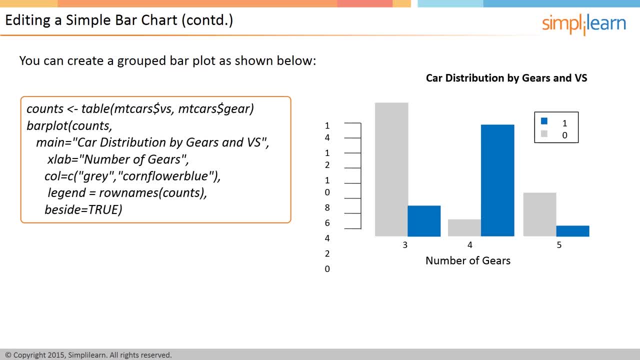 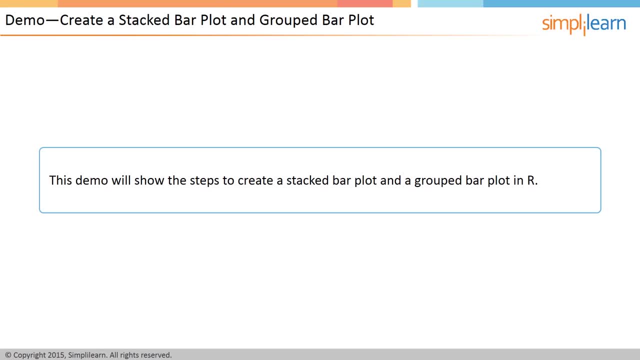 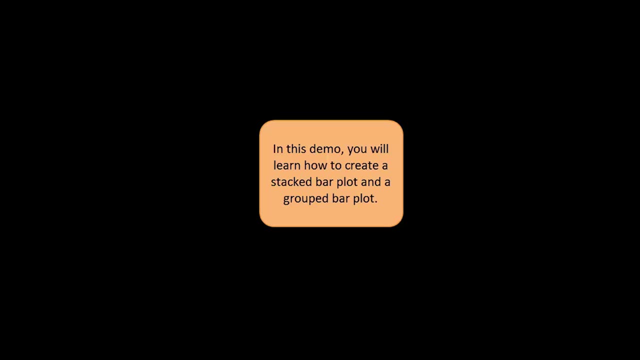 Here you use the row names function to set the legend which will set or retrieve the names of rows or columns of a matrix-like object. In this demo we'll show the steps to create a stacked bar plot and a grouped bar plot in R. In this demo you'll learn how to create a. 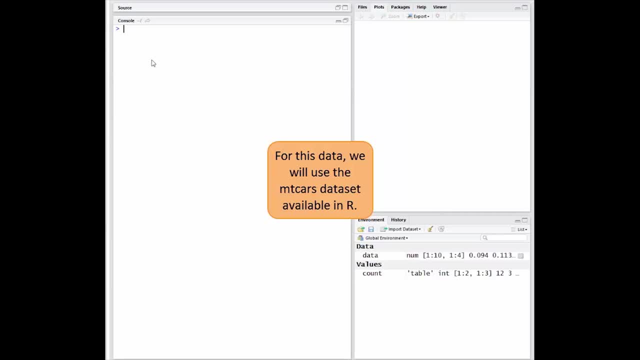 stacked bar plot and a grouped bar plot in R. You can create a group bar plot in R. You can also create a group bar plot in R In this. For this data we'll use the mtcars dataset available in R. For a stacked barplot and a grouped barplot we'll have to create a table like data from the mtcars dataset using the table function. 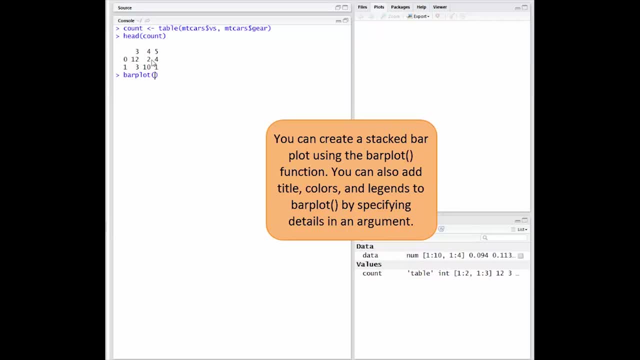 You can create a stacked barplot using the barplot function. You can also add title colors and legends to barplot by specifying details in an argument. You can create a grouped barplot by specifying beside equals true as an argument to the barplot function. 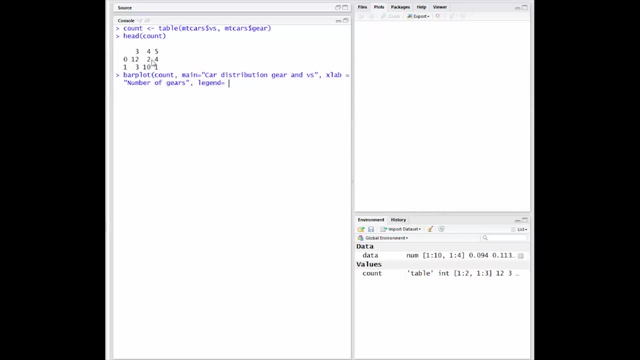 For a stacked barplot, we'll have to specify by adding a name. If we choose to add a name, we'll have to create a Money ID. In this case, we'll create a Money ID And this is the Money ID we created. 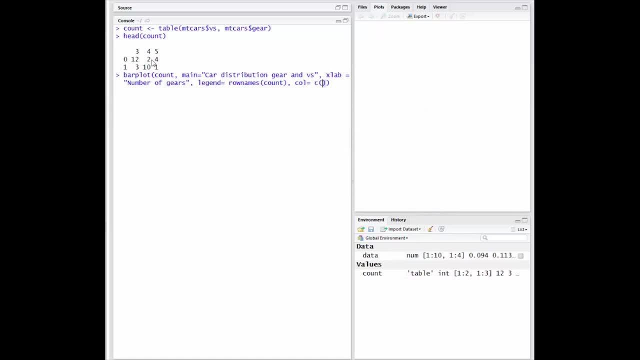 For a stacked barplot, we'll use the mtcars dataset as an example. For a stacked barplot, we'll use the mtcars dataset. In the same way, we can create a range of variables as the answers add To create the graph. we'll use the mtcars dataset as an example. 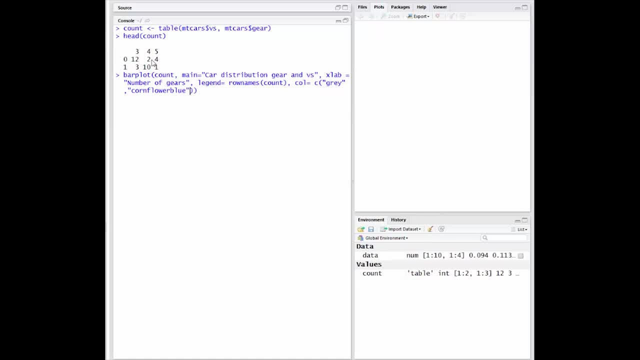 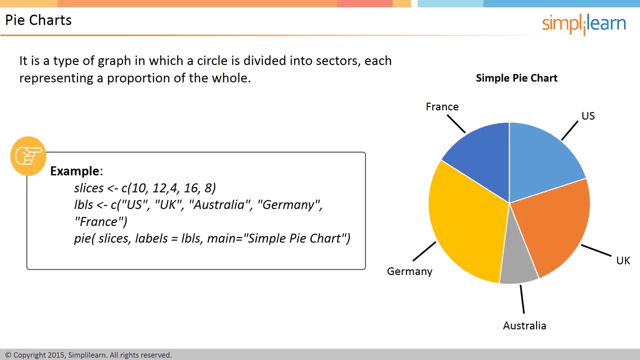 To create a barplot. we'll add a value to the slide For more options or help: document type: the given command in the console. Pie chart is a type of graph in which a circle is divided into sectors, each representing a proportion of the whole. 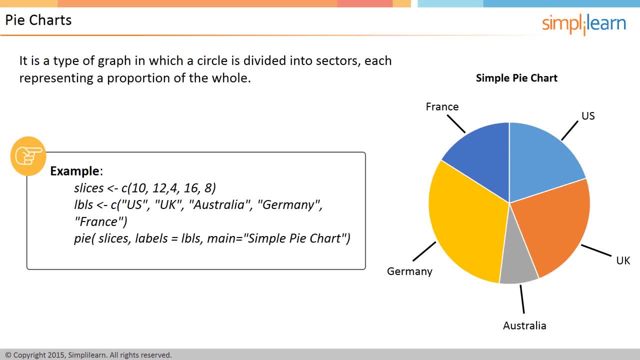 Pie charts are not as popular as dot plots or bar charts. in R You can create pie charts using the function. pi equals Here. x is a vector of non-negative numerical quantities. The value of x indicates the area of a pie slice. Labels are character strings or expressions that give names to vectors. 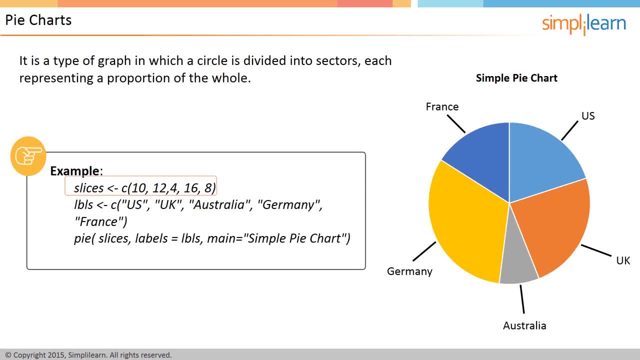 The example shown here. you first create the slices vector which contains numbers 10,, 12,, 4,, 16 and 8.. LBLS is the labels vector. Then you pass both these vectors to the pie function as parameters To set the overall title for the plot. you pass main as a parameter. 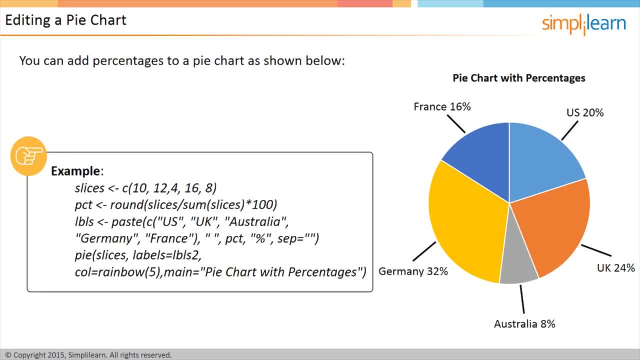 In this screen you can see how percentages can be added to the pie chart. In the given example, out of the data vector you can create the PCT vector and the character vector LBLS to add actual labels to the slices, To paste data to the pie. 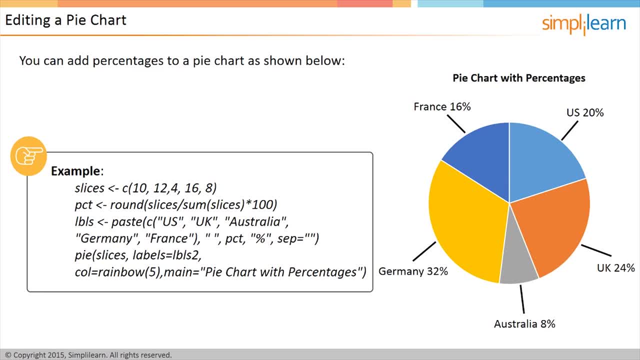 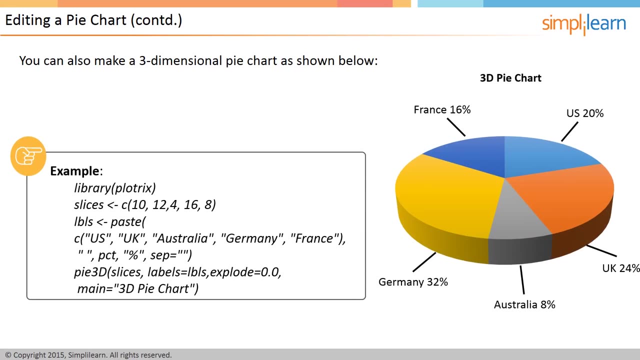 The labels vector and add the percentage sign. you use the paste function. Another character vector call helps fill in or shade the pie slices. Let's now see how you can create a three-dimensional pie chart. Using the plot tricks package, which has the pie 3D function, you can produce 3D representations. 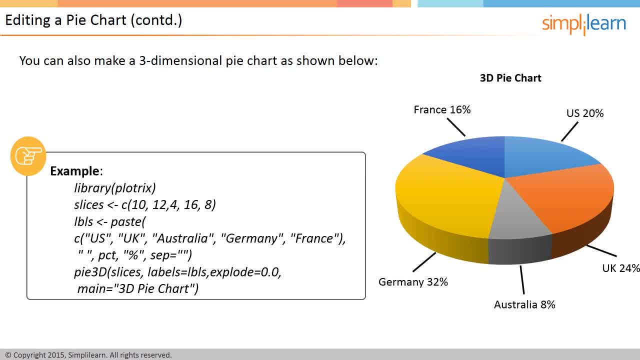 of pie charts. There is an explode parameter that enables the pieces to be separated on the chart. However, you first have to install the plot tricks package, Select it from the plot beginning하 and reference it using the library function install Prozentiles. 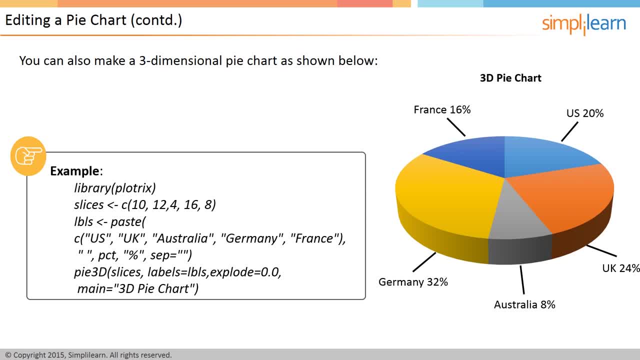 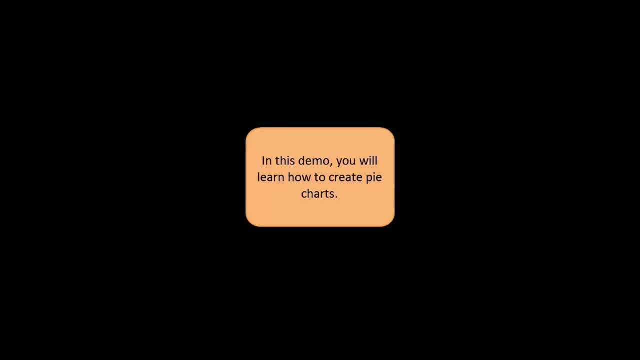 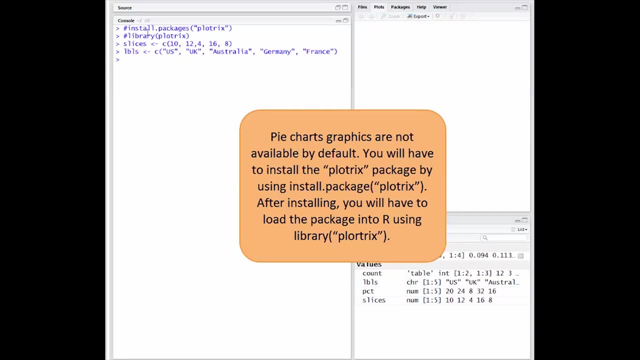 ion demain begging to be splitted into a cell alone. create a pie chart. desta demo will show the steps to create a pie chart. In this demo, you will learn how to create pie charts. Pie chart graphics are not available by default. you'll have to install the plot tricks package. 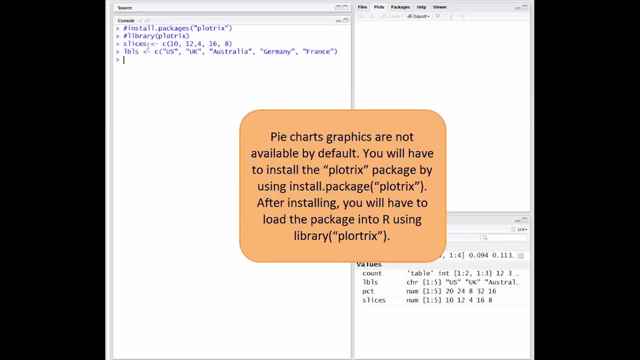 by using the given command. After installing, you'll have to load the package into R using the given command. This will take you three minutes. This demo is super interesting. Okay, 먹otypydit file For this demo. we'll create a custom dataset using vectors. 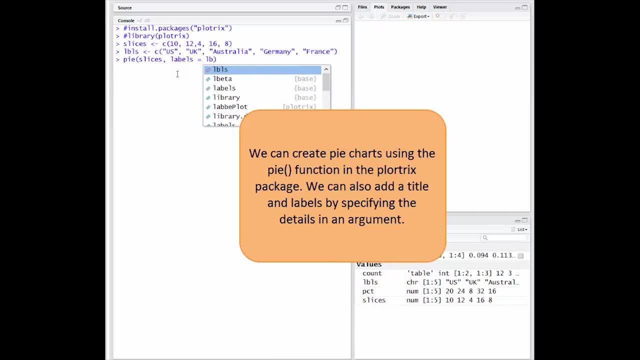 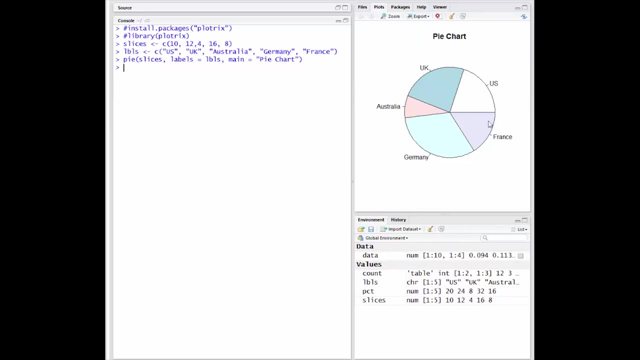 We can create pie charts using the pie function in the Plotrix package. We can also add a title and labels by specifying the details in an argument. We can specify the defined shooting time without needing to specify it, or we can tweak the target video. 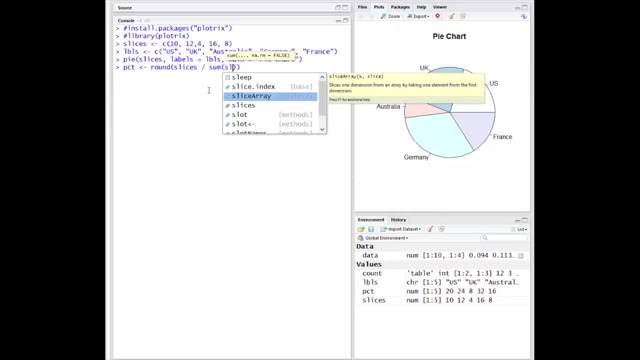 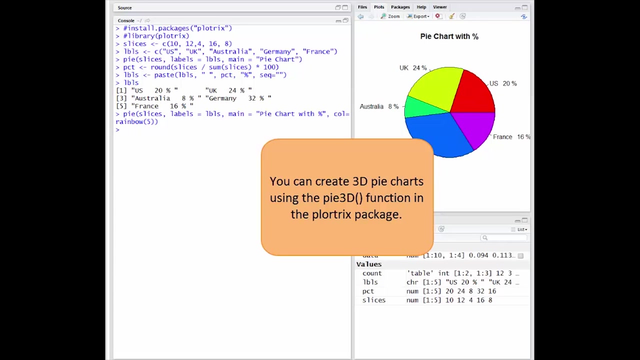 Here you can see we've getting a new diamond. Wait, a second right this time. there is also a little gap here between the two screens. This is a mistake. you You can create 3D pie charts using the pie3D function in the Plotrix package. 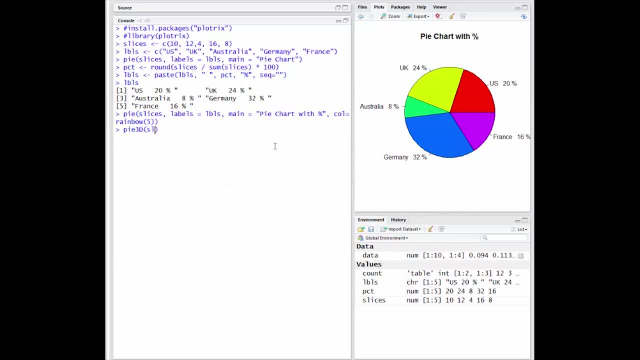 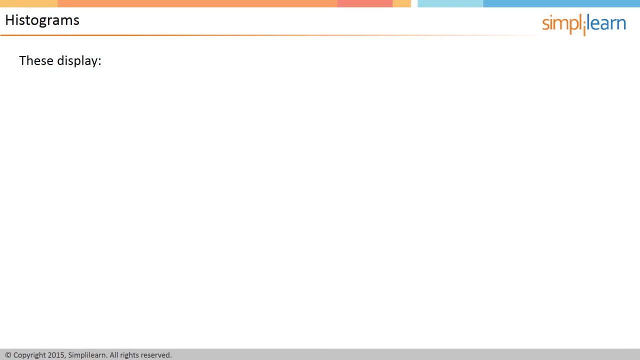 Thank you for watching For more options or help document type the given command in the console. Let's look at another visual representation of data distribution: the histogram. Histograms are a great way to get to know your data. A histogram has an x-axis, a y-axis and bars of different heights. 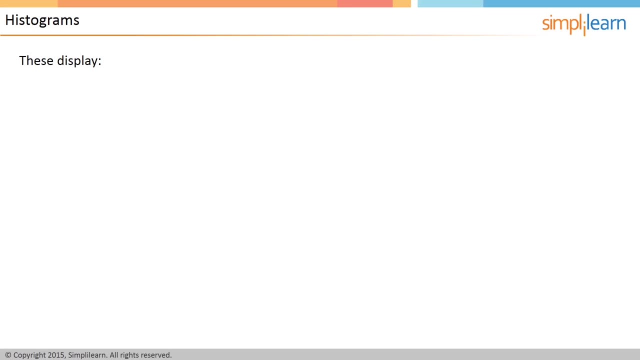 The bars group ranges of values or continuous categories on the x-axis and the y-axis shows how frequently the values on the x-axis occur in the data. They display the distribution of a continuous variable and the frequency of scores in each bin on the y-axis. 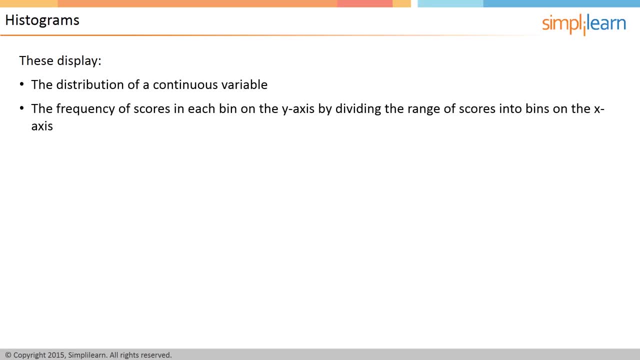 by dividing the range of scores into bins on the x-axis, As shown on the screen. the syntax for a histogram is hist in R. For a given set of data values, the generic function hist works out a histogram If plot equals true plothtml. 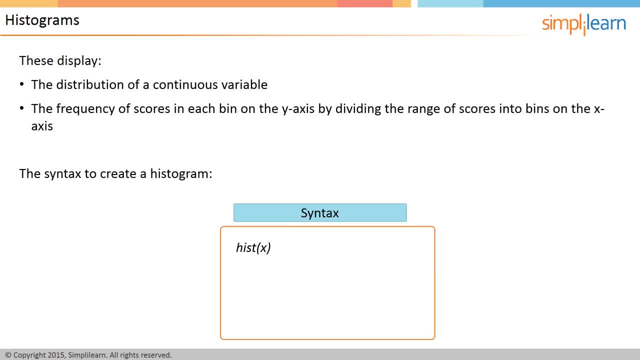 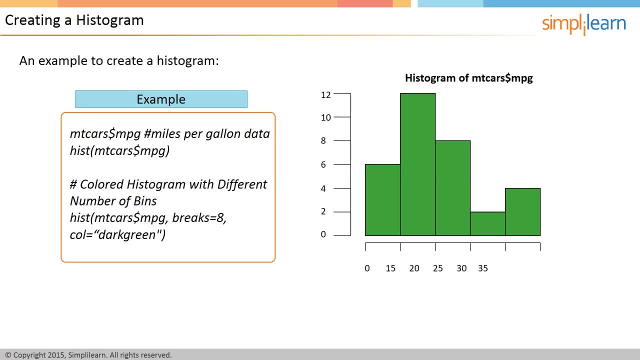 Histogram plots the resulting object of class Histogram before it's returned. You can create a histogram using the histx function where x is a vector of values for which you want to plot the histogram. Instead of frequencies, the option frequency equals false plots- probability density when you want a histogram of proportion. 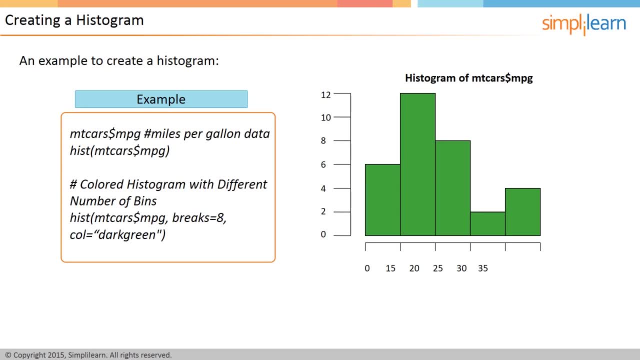 To control the number of bins, that is, bars, use the breaks equals controls option. The break argument helps you control the bin width along with the number of break points you desire. In the example shown on the screen, you can see histograms for dark green colored bins. 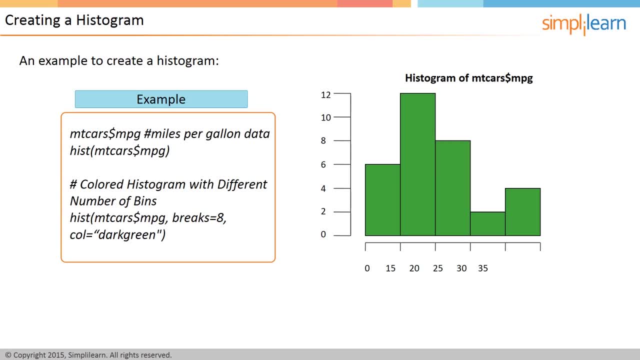 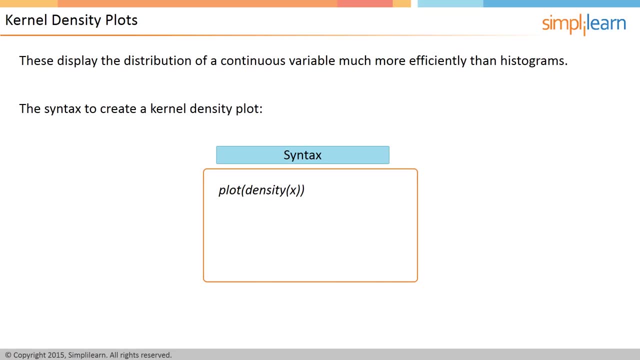 that indicate the miles per gallon or mpg value of the empty cars data set. A more effective way of visualizing numeric variable distribution. kernel density plots are created using the plotdensityx function. as shown on the screen Here, x is a density object. 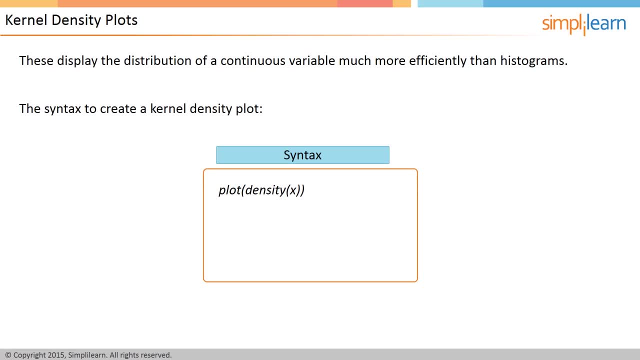 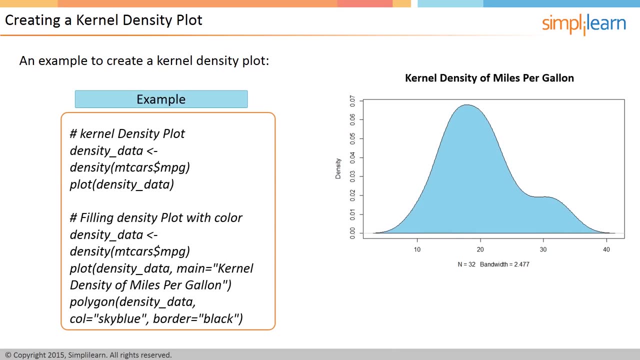 You can use the density function to compute the density parameter in plot. In the example shown in this slide, you can create a kernel density graph for the mileage per gallon or mpg of empty cars, data set by first calculating its density and then creating the graph. 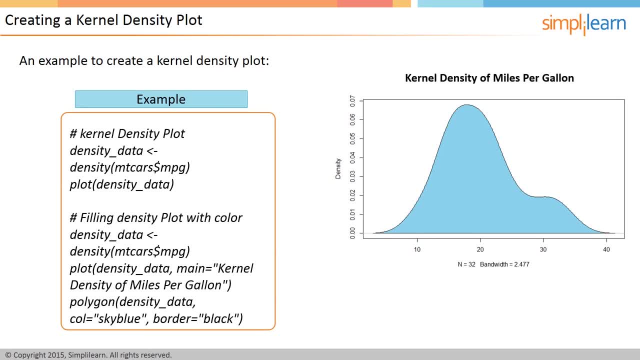 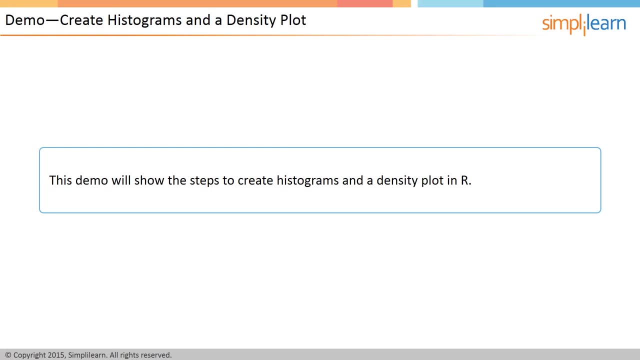 In the second figure use the polygon function for kernel density of the data. for mpg Vertices are given in x and colors of the area and the border are given by: color equals sky blue and border equals black respectively. This demo will show the steps to create a histogram and density plot in R. 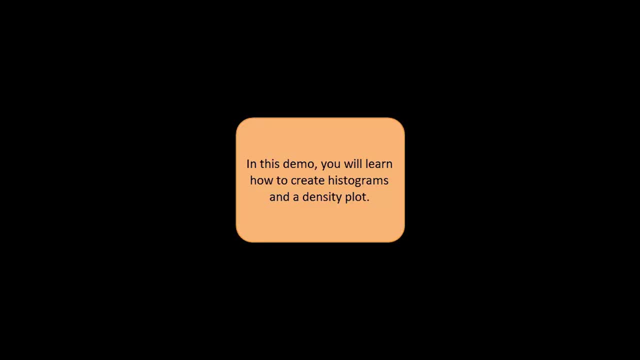 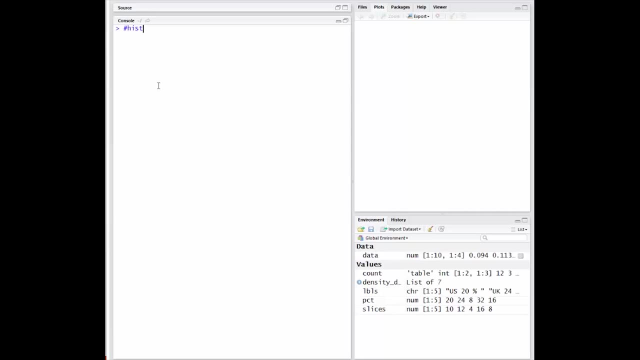 In this demo, you'll learn how to create histograms and a density plot. For this demo, we'll use the empty cars data set available in R. Histograms can be created in any more than one audi edits on R and we'll use it to make histograms. 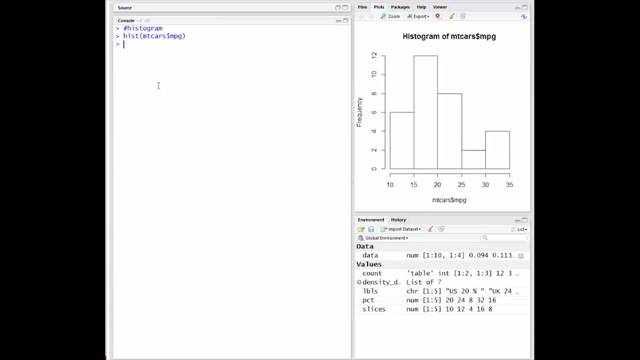 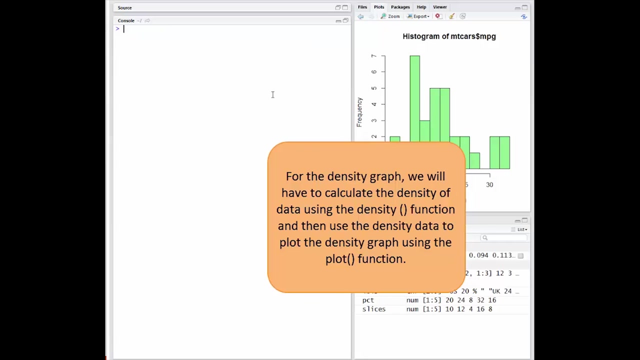 using the HIST function. You can also specify the number of bins and the color of bin as arguments to the HIST function For the density graph. we'll have to calculate the density of data using the density function and then use the density data to plot the density graph using the plot function. 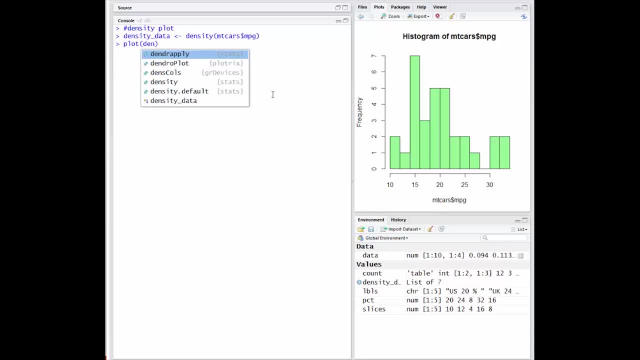 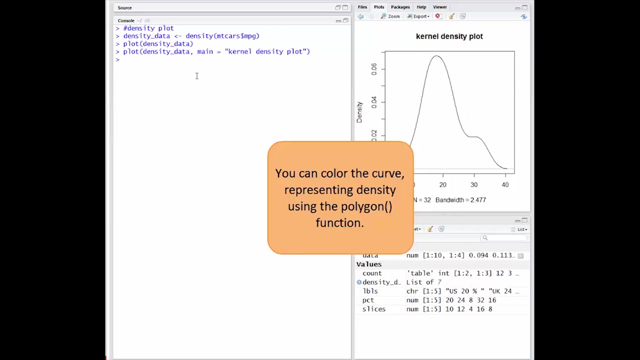 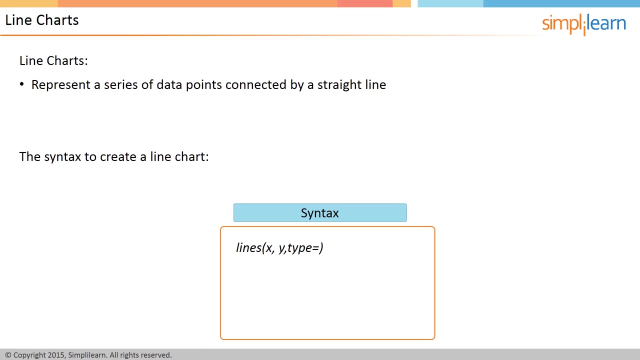 You can color the curve representing density using the polygon function For more options or help document type the given commands in the comment section. Line charts represent a series of data points, called markers, connected by a straight line. This type of graphical visualization is typically used to display data that changes over time. 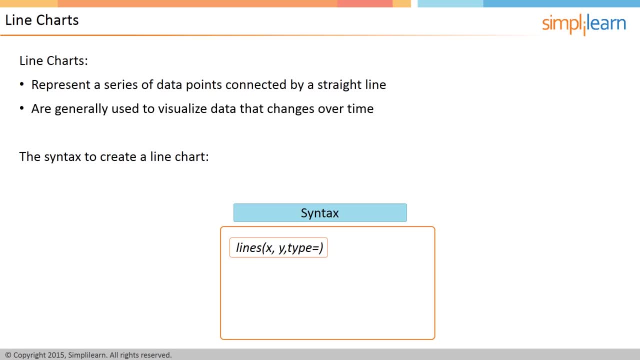 As shown on the screen, the syntax for a line chart is lines: x, y. type equals where x and y are coordinates of the points. Type indicates the type of plot to be drawn, say L for line and P for points, or B for. 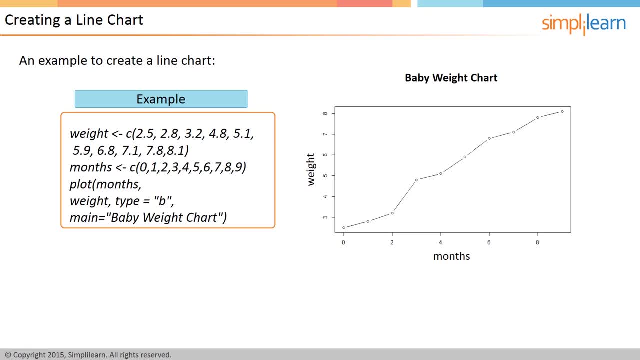 points. Let's now look at an example of a line chart. In the code shown in this slide, you can create weight and months vectors and then plot a line and points graph together. by calling the plot function, These two vectors are passed as parameters, along with main to set the title of the graph. 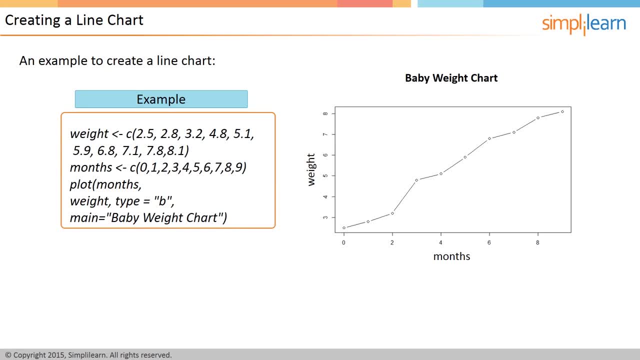 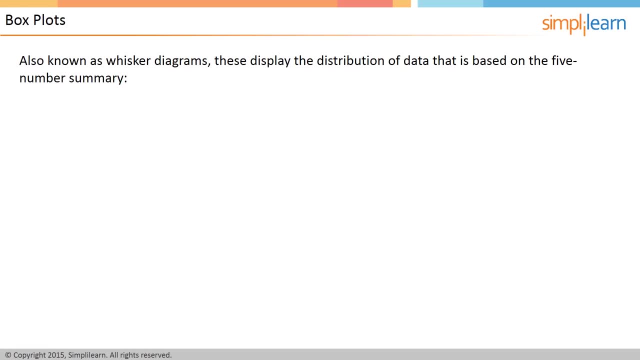 as baby weight chart, Also known as whisker diagrams. box plots display the distribution of data that is based on the 5-point graph. The data set is divided into the first quartile, 25th percentile. median, 50th percentile. 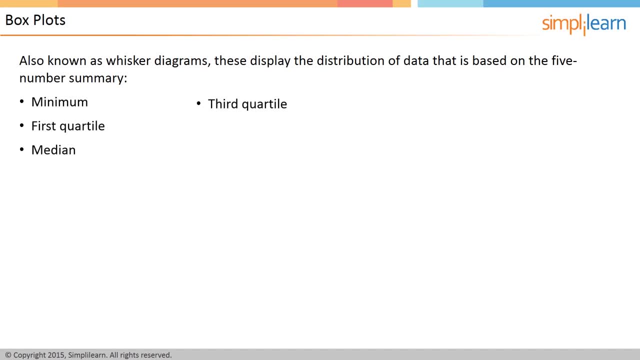 third quartile, 75th percentile and maximum largest value in the data set. Data is broken into four quartiles in box and whisker plots, and each quartile has the same number of data values. Although these plots do not display the frequency, they show where the middle of the data is. 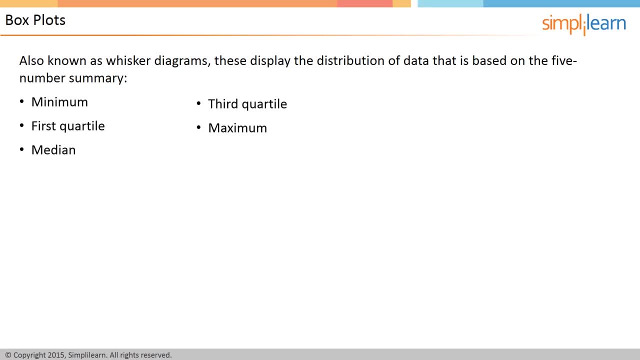 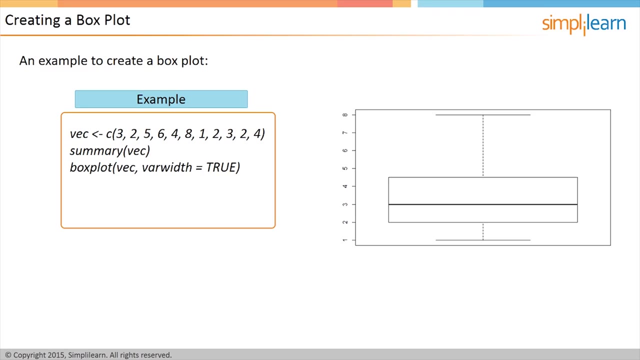 a feature that is really useful if you want to analyze the skewness of your data. The syntax to create a box plot is shown on the screen: Box plot data. A box can be created either for individual variables or for variables by group. As shown on the screen, the syntax is: box plot: x data equals where x is a formula and. 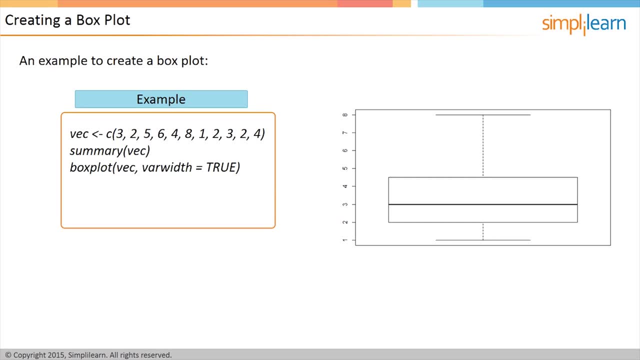 data equals denotes the data frame providing the data To make the widths of the box plots. you can create a box plot x. data equals To make the box plot proportional to the square roots of the number of observations in the sample. use var width equals true. 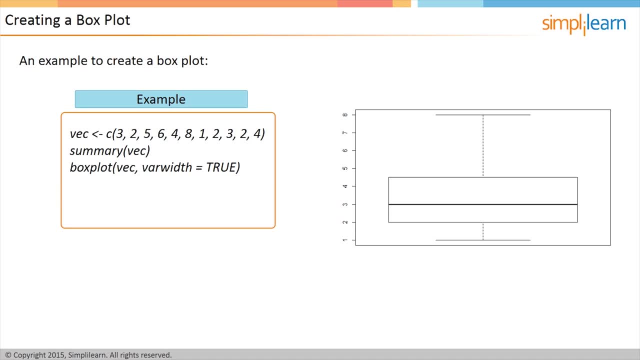 With horizontal equals: true, you can reverse the orientation of the axis. Default: false means the box plots are vertical. In the code shown here, a vector of numbers was created and the summary function called to print the values of the following variables: Minimum first quartile. 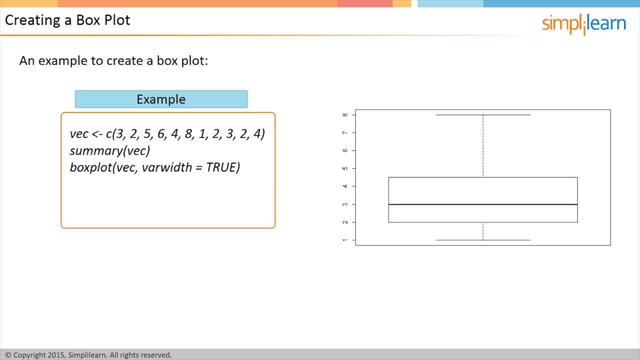 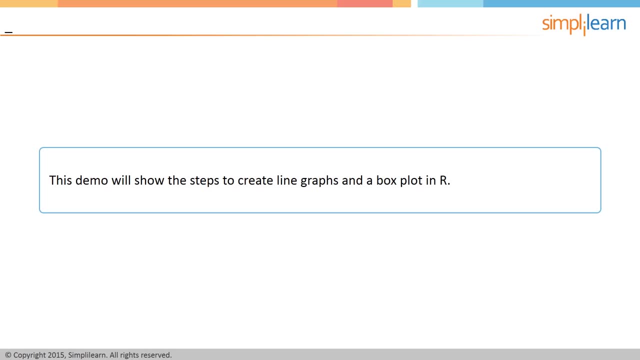 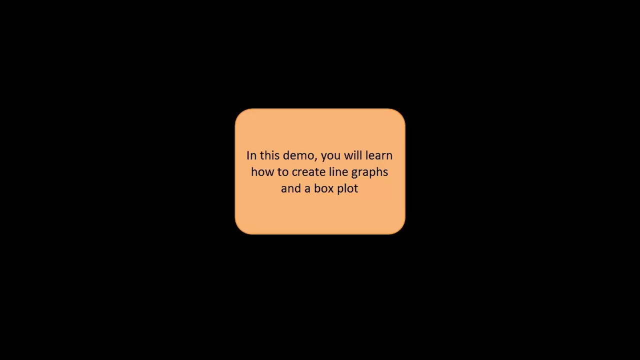 Median Mean, third quartile Maximum. Then the box plot function was used to display the box plot for the vector of numbers. This demo will show the steps to create line graphs and a box plot in R. In this demo, you'll learn how to create line graphs and a box plot. 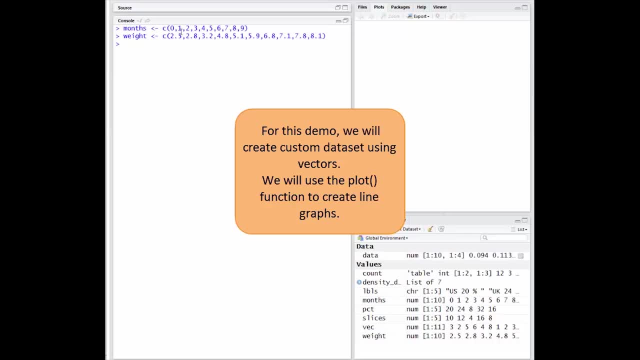 For this demo we'll create custom data set using vectors. We'll use the plot function to create line graphs. To create line graphs, we use the plot function, which is linked to the set in R. Points in a line graph can be connected by specifying type: equals b as an argument in. 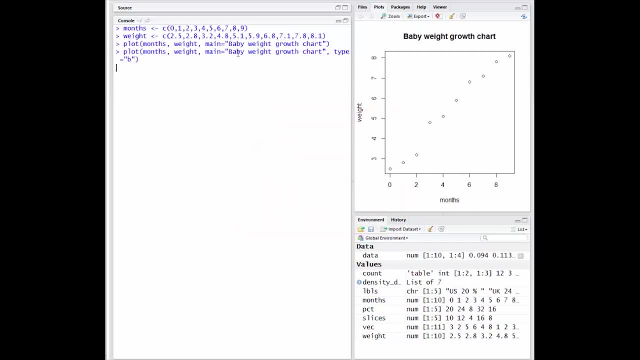 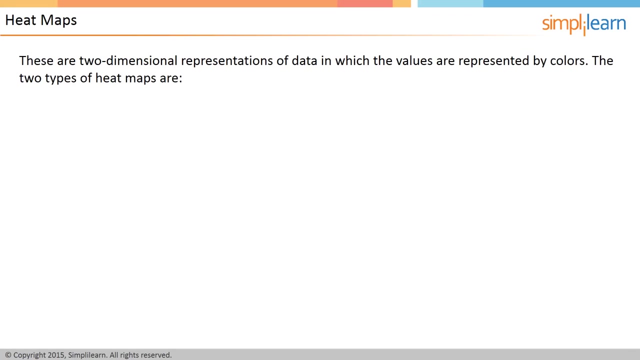 the plot function. We can create Box Plot using the Box Plot function. We can create Box Plot using the Box Plot function For more options or help document type. the given commands in the console Heatmaps are two-dimensional representations of data in which the values are represented by colors. 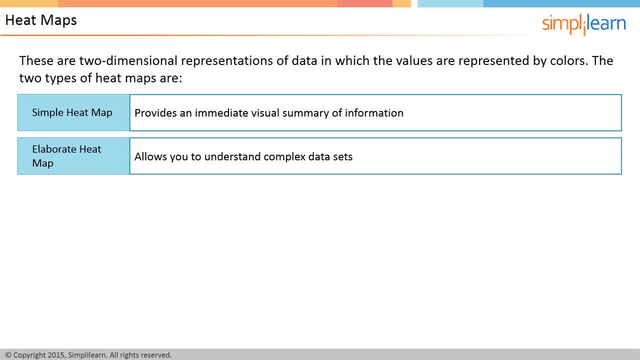 The two types of heatmaps are simple and elaborate heatmaps. A simple heatmap provides an immediate visual summary of information. An elaborate heatmap allows you to understand complex data sets. Rows and columns can be clustered in a heatmap and the result of the hierarchical clustering computation is shown as a dendrogram in the heatmap. 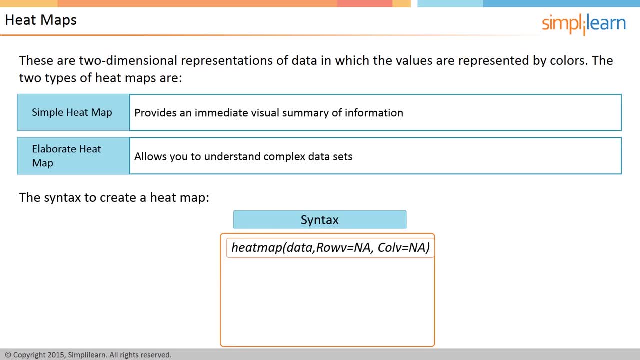 As shown on the screen, the syntax to create a heatmap is heatmap data. row V equals NA, column V equals NA. Here, row V and column V decide if and how row and column dendrograms should be calculated or reordered. Data refers to the matrix of values. 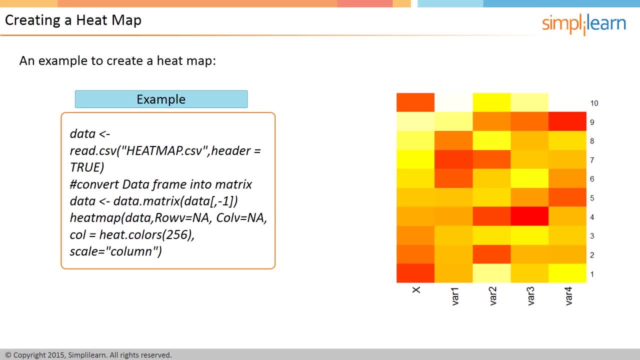 that have to be calculated or reordered. Data refers to the matrix of values that have to be plotted. Let's look at an example that shows you how to create a heatmap. In the code shown here, you can create a data frame by reading data from a CSV file. 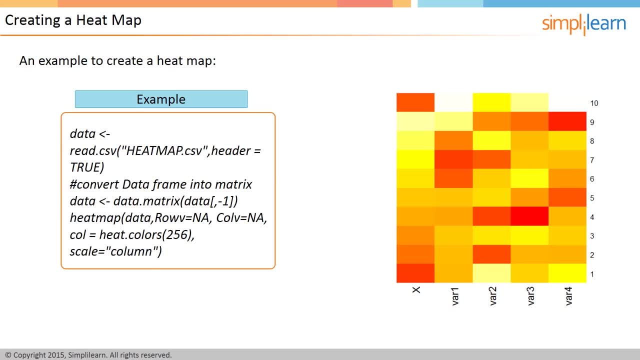 and converting it to a data frame before passing it to the heatmap function. Besides, data, row V and column V as not applicable, color as 256, and scale as columns to plot a heatmap graph are passed to the heatmap function. This demo will show you how to create a heatmap and how to plot a heatmap graph. 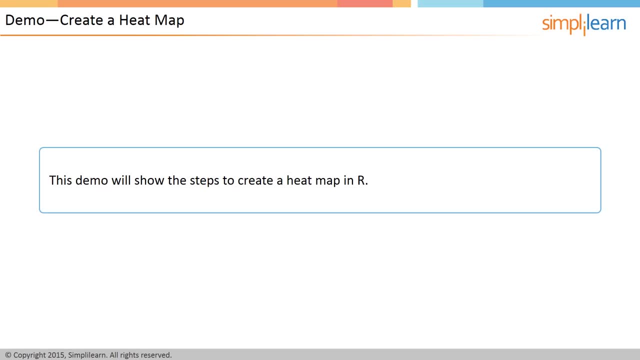 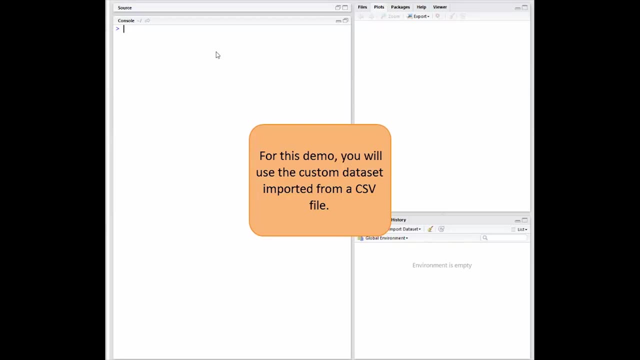 This demo will show the steps to create a heatmap in R. In this demo you'll learn how to create a heatmap. For this demo you'll use the custom dataset imported from a CSV file. The code starts at the input. The data will then be taken to an output, to the main function for the heatmap. 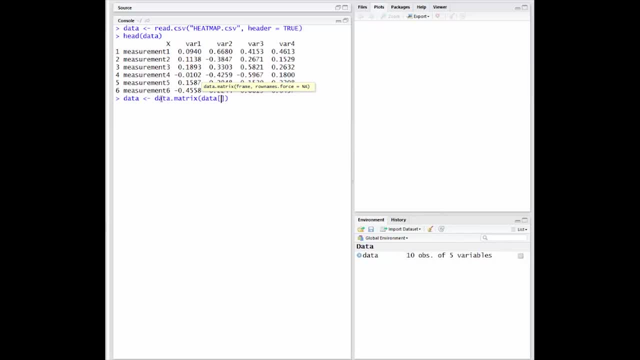 The heatmap can be constructed using the heatmap function. You can then specify the color and scale details as arguments to the heatmap function. In the last section I explained the heatmap function and how to use it. Thanks for watching. Take care everyone. 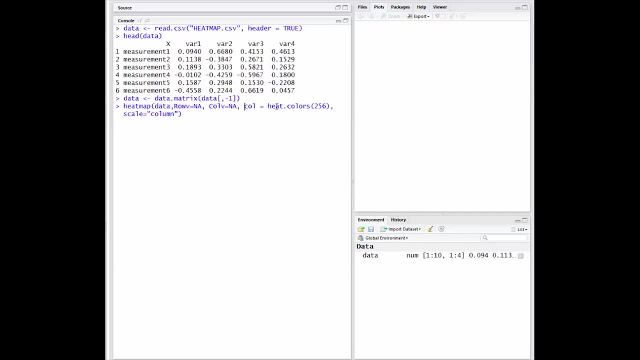 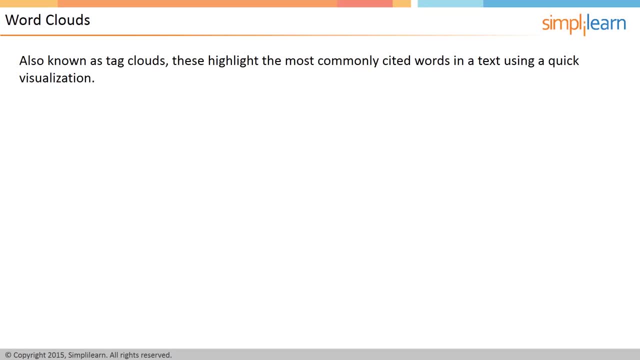 Also known as tag clouds or text clouds. word clouds highlight the most commonly cited words in a text. using a quick visualization, Creating a word cloud in R is relatively simple using a text mining package and word cloud generator package. As shown on the screen. to create a word cloud, use the syntax word cloud words equal data. 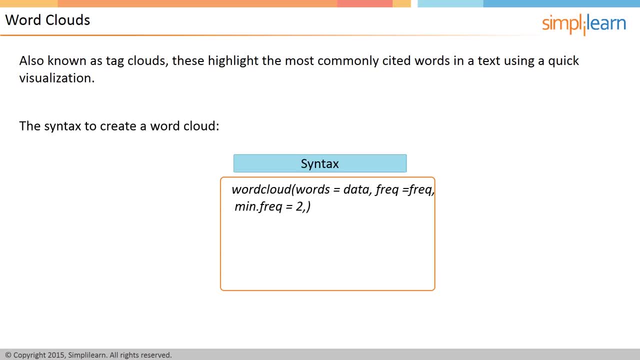 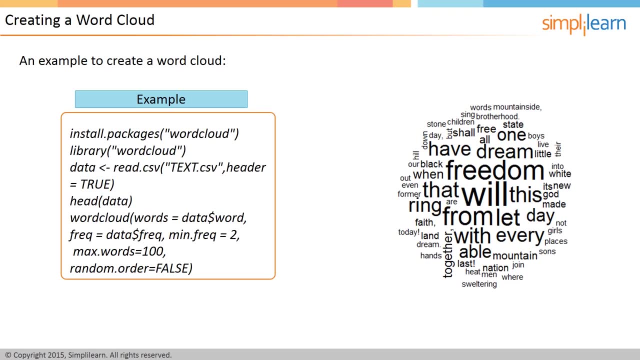 frequency equals frequency, minfrequency equals 2, etc. You need to install the word cloud package into the R environment using the installpackages word count and library word count commands. In the example on this screen, text data is read from a CSV file and the word count 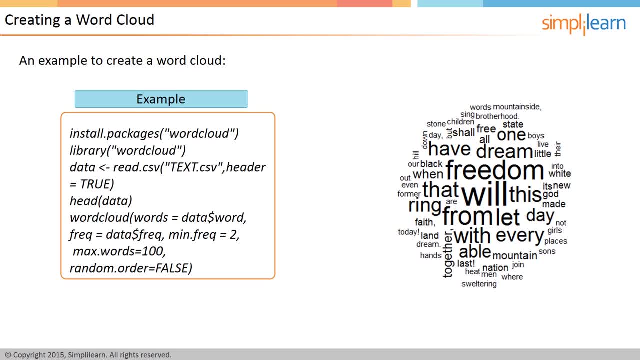 graph is plotted using the word count function. Passwords, frequency: minfrequency as 2, maxwords as 100, and randomorder as false. The minimumfrequency argument specifies the minimum frequency below which words that have a frequency lower than that value will not be plotted. 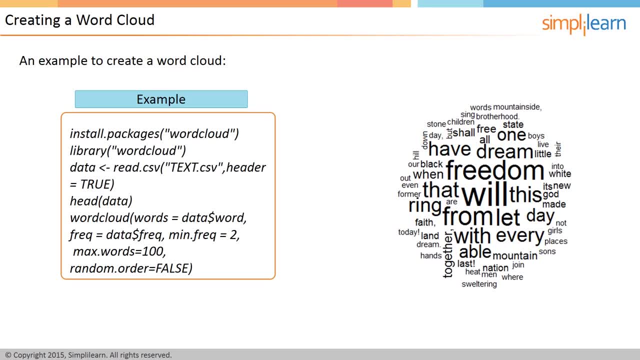 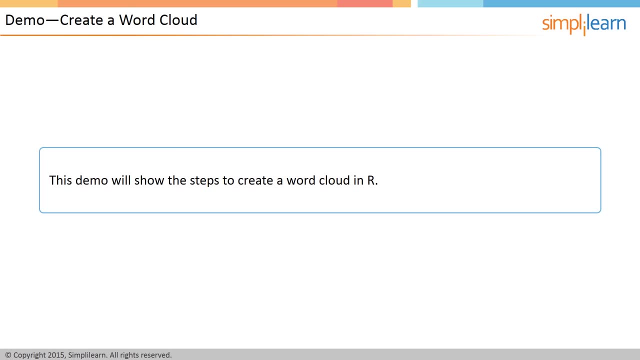 The maximum number of words to be plotted are determined by the minimumfrequency. Randomorder means that the words will be plotted in a random order. If false, the words are plotted in decreasing frequency. This demo will show the steps to create a word cloud in R. 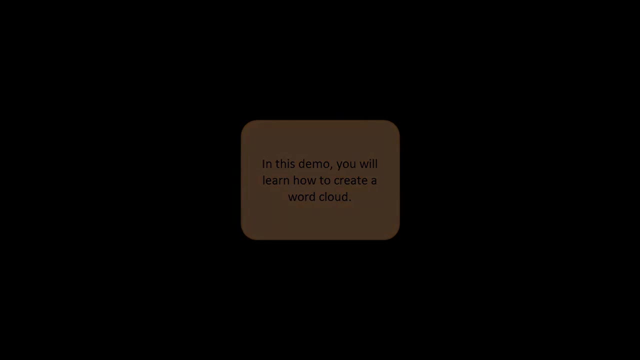 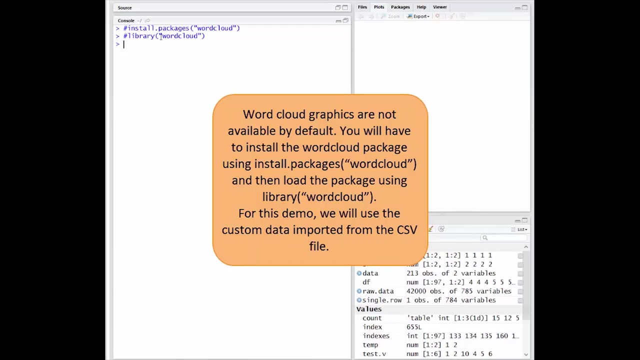 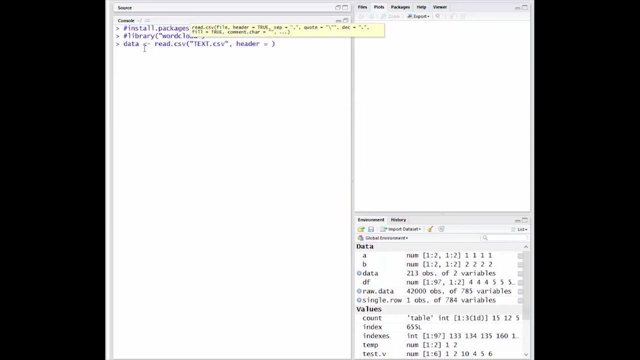 In this demo, you'll learn how to create a word cloud. Word cloud graphics are not available by default. You'll have to install the word cloud package using the given command And then load the package using the other command. For this demo, we'll use the custom data imported from the CSV file. 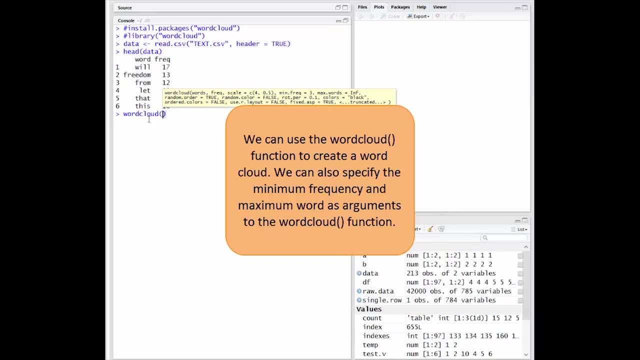 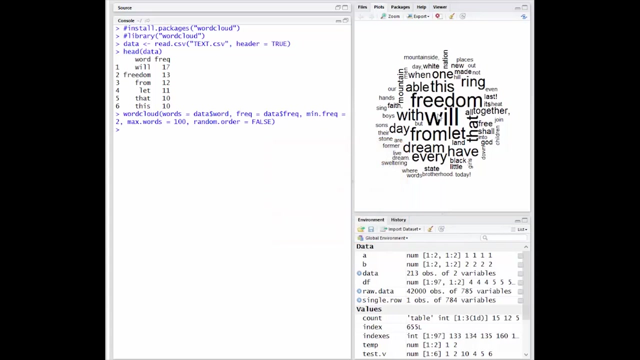 We can use the word cloud function to create a word cloud. We can also specify the minfrequency and maxword as arguments to the word cloud function For more options and help document type the given command in the console. Let's now take a look at the various file formats for saving your plots. 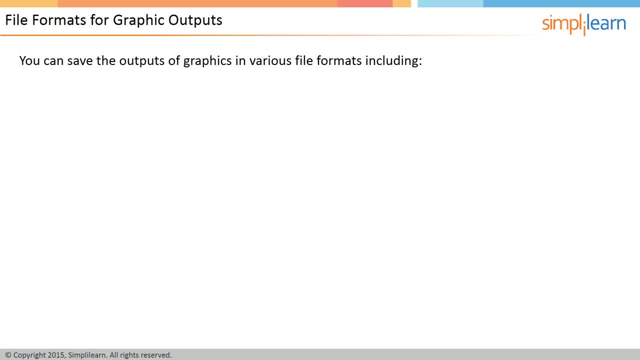 R supports several graphic formats and runs on different operating systems. Consequently, there are many formats to choose from, depending on what you want to do with the graph, How you connect, What you use remotely or locally, And what operating system you use. A few of the available formats are as follows: 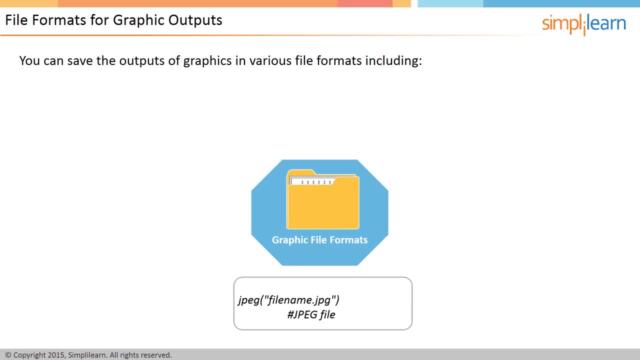 JPEG: Doesn't resize and can be used anywhere. PDF: Easily resizable and is the best choice with PDF. latex. PNG: Doesn't resize and can be used anywhere. WMF: Easily resizable and works on Windows only- Best choice with Word. 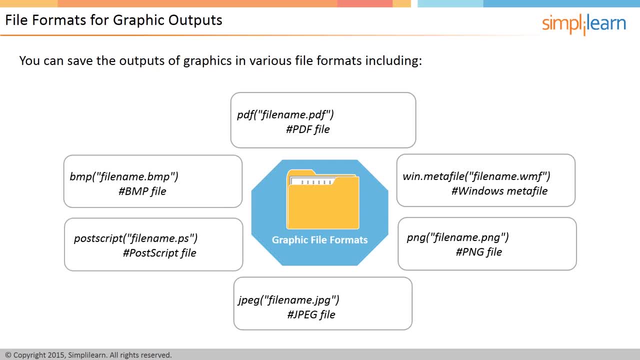 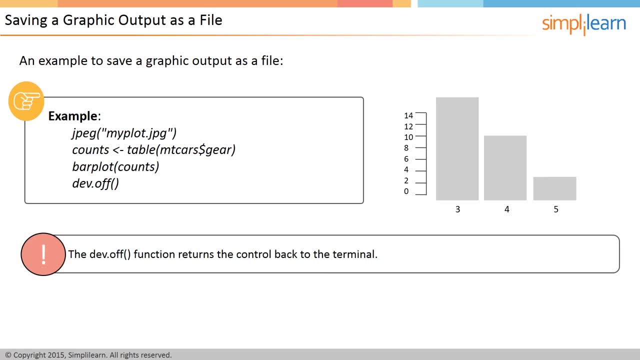 PostScript, Easily resizable and is the best choice with OpenOffice and Latex. On the slide you can see an example to save a graphic output as a file. Regardless of the way you connect or the type of operating system you use, the general method. 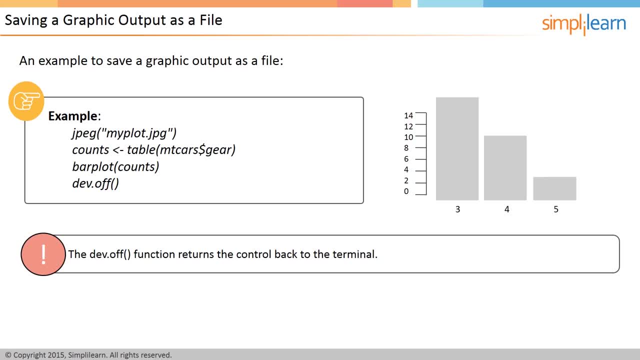 that will work on any computer that has R. involves the following steps: Select the file format you want. for example, if you want to save your plot as a JPEG file, Use the JPEG driver. Use the JPEG driver. Use the JPEG driver. 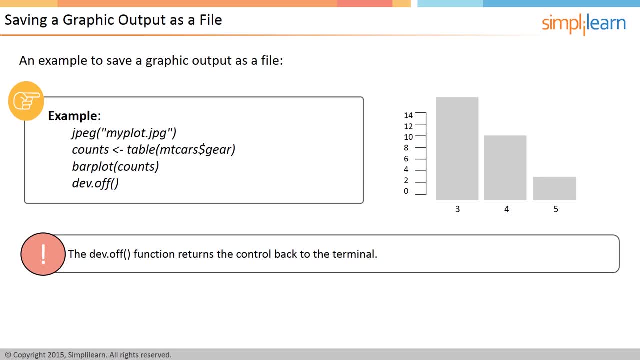 Or use the name of the file that you will use to save the graph. Note that your plot will be stored relative to the current directory, which can be found by typing git wd at the R prompt. Entering your plotting commands next will save those to a file. 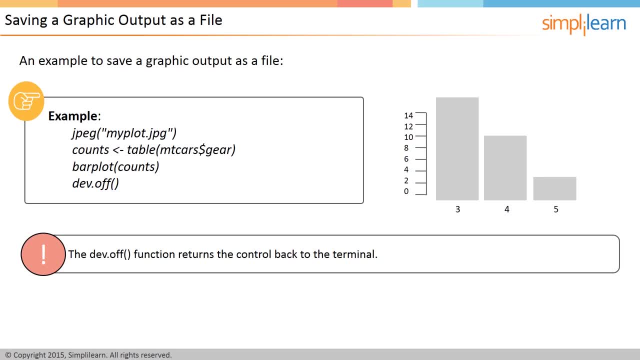 Then use the devoff command to close the file. Either you will get a partial plot or nothing. in case you fail to enter the devoff command after you are done with plotting commands, Save theη size on fcp2 file. Who's there? 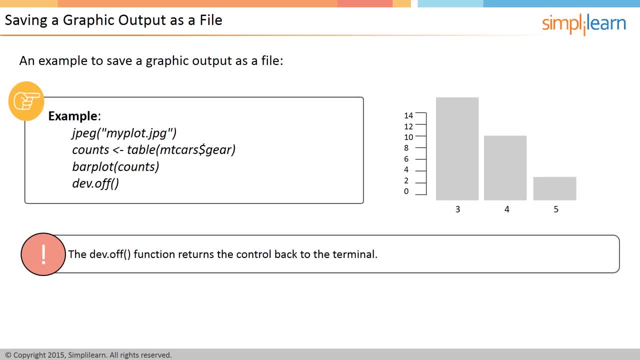 If you want to save a JPEG file called myplotjpg, containing a bar graph, you will type the commands as shown on the screen Recalling the example from the previous screen. you will see that you need to re-enter the commands to save your plot to a file after making a plot to the screen. 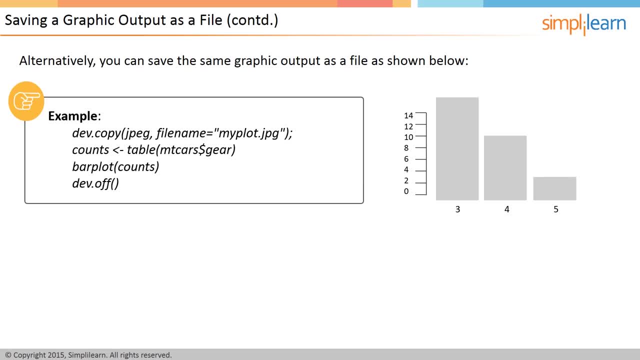 However, in R there is another command, devcopy, which will copy the contents of the graph window to a file without the hassle of re-entering the commands. In this approach, produce the graph as you usually do, and then call devcopy, along with the arguments that are appropriate to the driver. 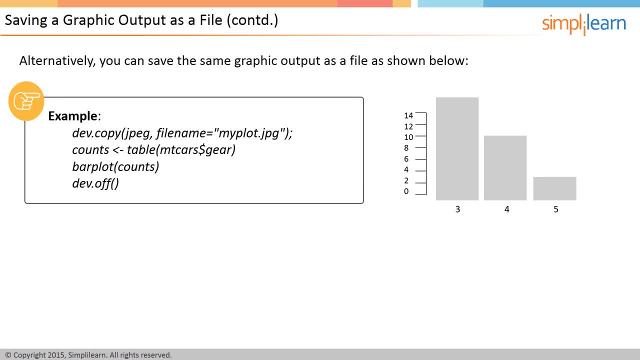 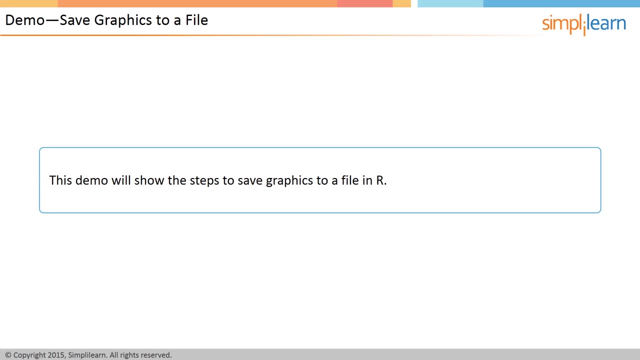 For example, to create a myplotjpg file from a graph shown by R, type the commands shown on the screen. Until you call devoff, the plot isn't actually written. This demo will show the steps to save graphics to a file in R. 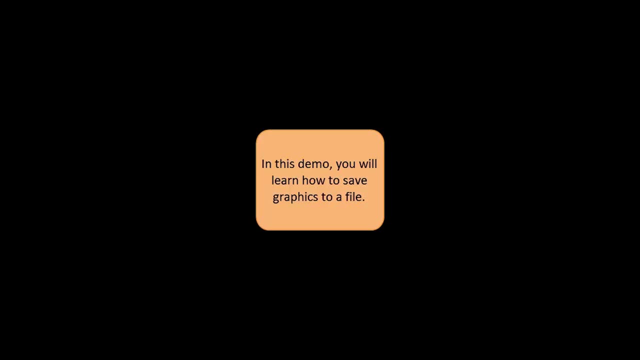 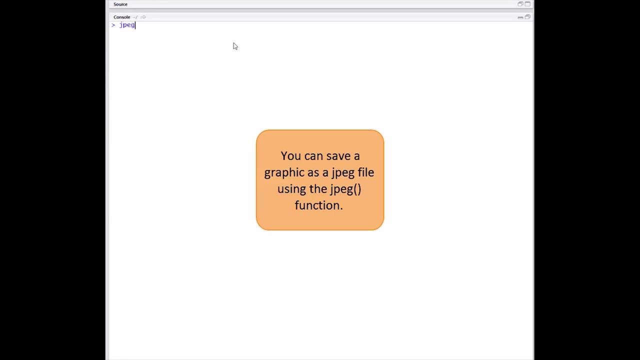 In this demo, you'll learn how to save graphics to a file. You can save a graphic as a JPEG file using the JPEG function. You can also save a JPEG file using the JPEG function. You'll also have to use the devoff function to return the control to the console back again. 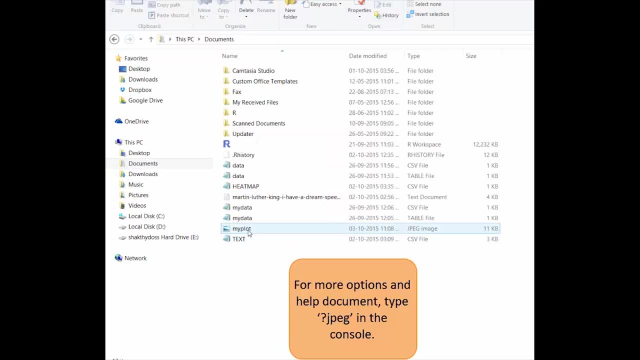 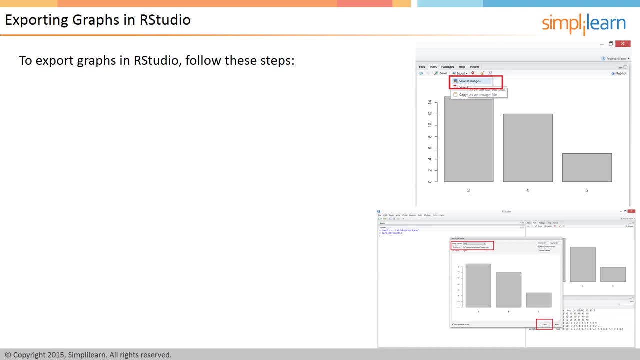 For more options and help document, type the given command in the console. In this screen you can see that the control is now saved. In this screen let's see how you can export graphs in RStudio. Follow these steps to export graphs in RStudio, a powerful interface for R. 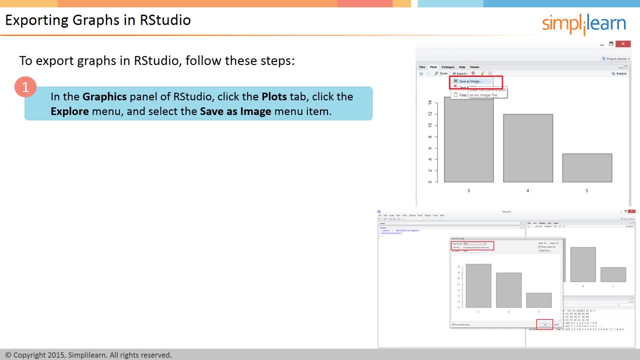 In the Graphics panel of RStudio. click the Plots tab, Click the Explore menu and select the Save as Image menu item. The Save Image window is displayed. Select the image format and directory to save the file. Click the Save button. Follow these steps to export graphs as PDFs in RStudio. 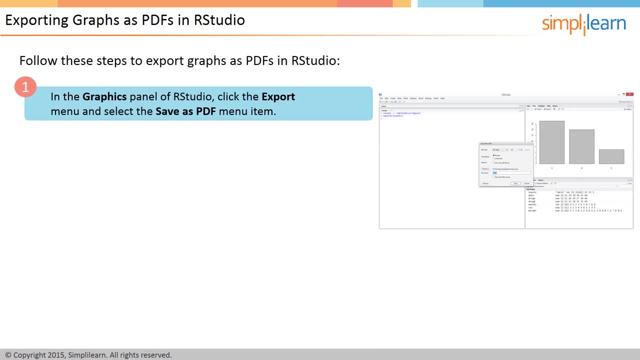 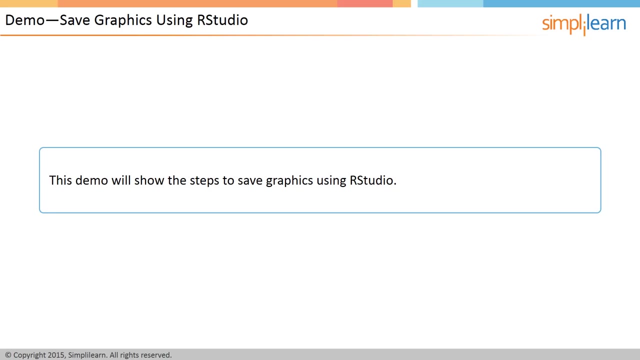 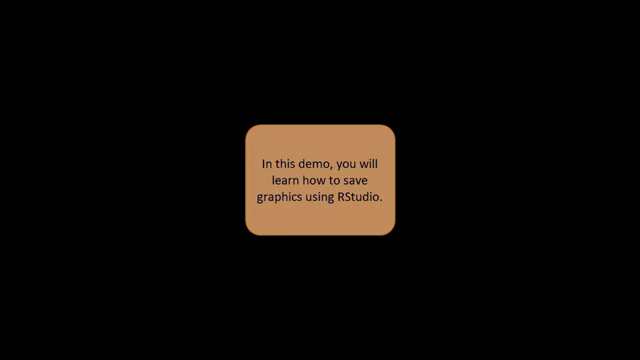 In the Graphics panel of RStudio, click the Export menu and select the Save as PDF menu item. Select the directory to save the file. Click the Save button. This demo will show the steps to save graphics using RStudio. In this demo, you'll learn how to save graphics using RStudio. 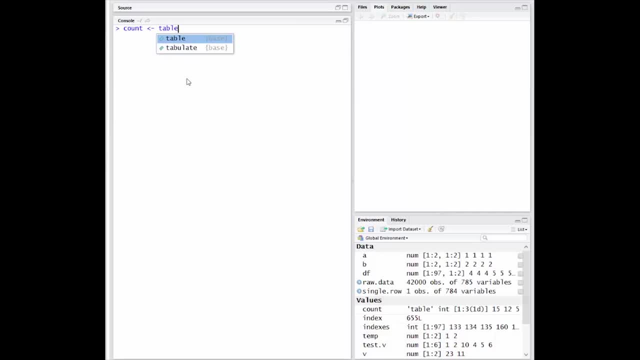 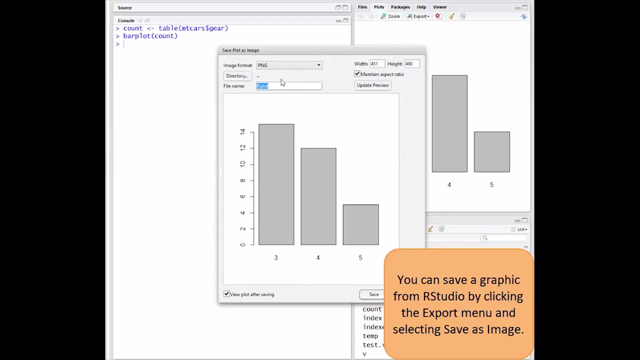 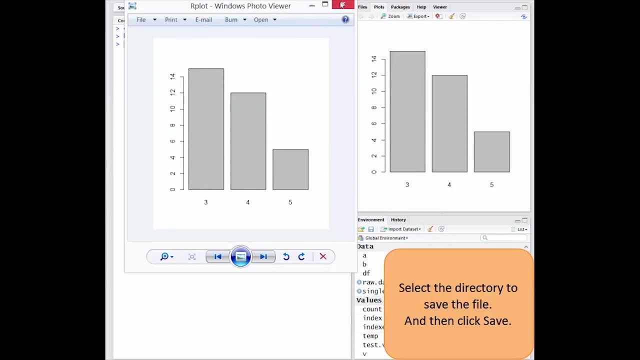 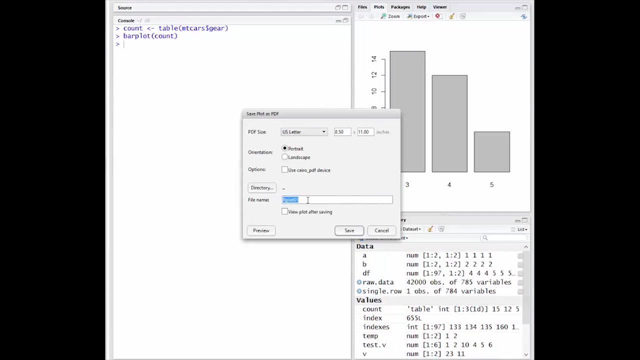 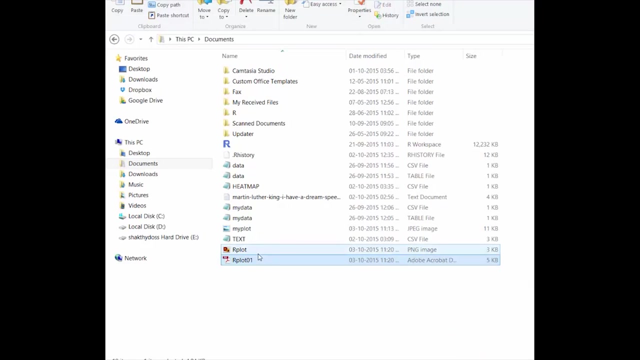 You can save a graphic from RStudio by clicking the Export menu and selecting Save As Image. You can save a graphic from RStudio by clicking the Export menu and selecting Save As Image. Select the directory to save the file. to save the file and then click Save.